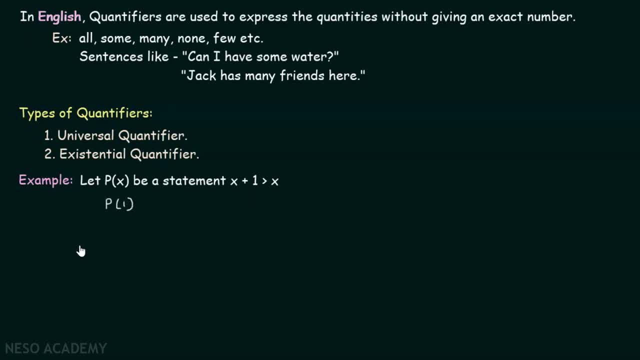 I would like to ask one question: What is the truth value for P1?? P1 will be definitely one plus one greater than x, Or I can replace this x by one. Then this will be equal to two greater than one, And this is true. 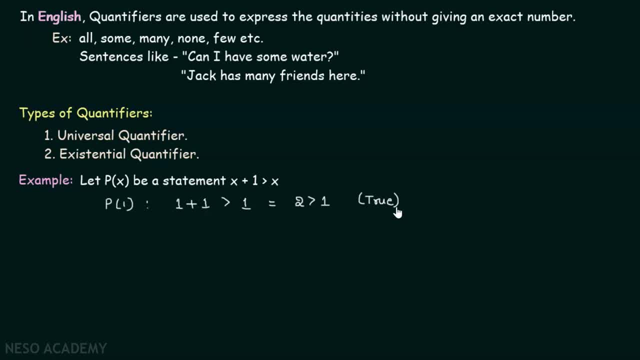 So two is greater than one, and that is why the truth value of P1 will be true. What will be the truth value for P2?? P2 will be two plus one greater than two, Which is finally equal to three greater than two. 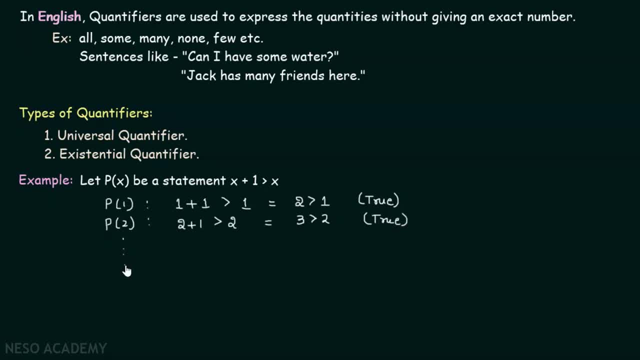 And yes, this is also true And this continues in the same way, right? Actually, it is true for all positive integers. Let me tell you, Px is true for all positive integers x. This should be well noted, that, whatever the positive integer you will take, 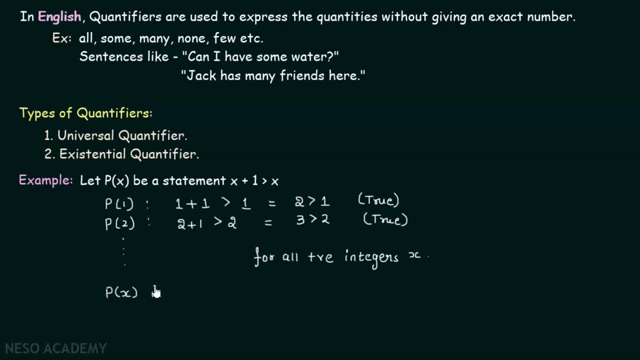 Px will always be true. So I can say that Px is true for all positive integers x. Or in other words, I can say for all x, Px. This is another way of saying this sentence. This particular notation is called for all. 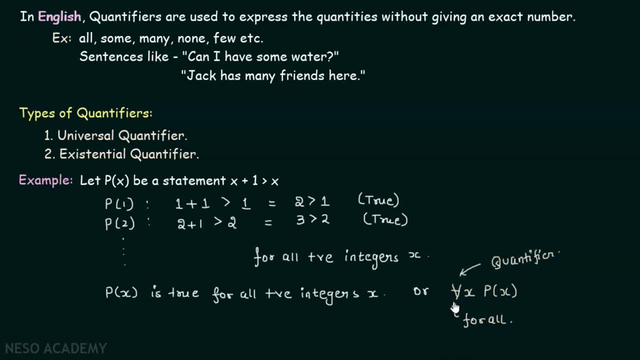 This is the quantifier we are talking about. We will use this quantifier to denote that Px is true for all positive integers x. Here x represents positive integers, Px is our predicate and this notation is called for. all Okay, we will use this notation. 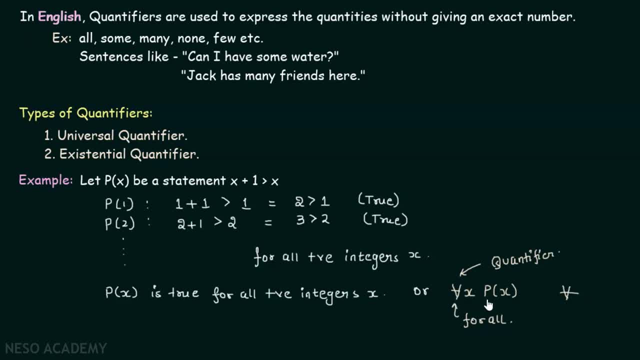 This represents for all, So we will put this in front of this: x- Px And we can read this: as for all x or for all positive integers: x? Px is true. I am repeating this once again: For all positive integers, x? Px is true. 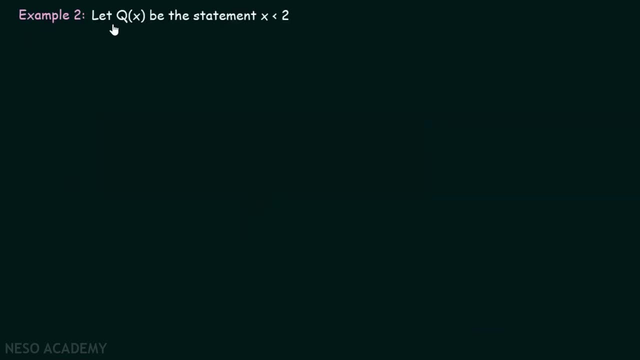 Now let's consider one more example. Let Qx be the statement x less than 2.. Let's do the same procedure once again. What is the truth value for Q1?? I would like to ask this question again: What is the truth value for Q1?? 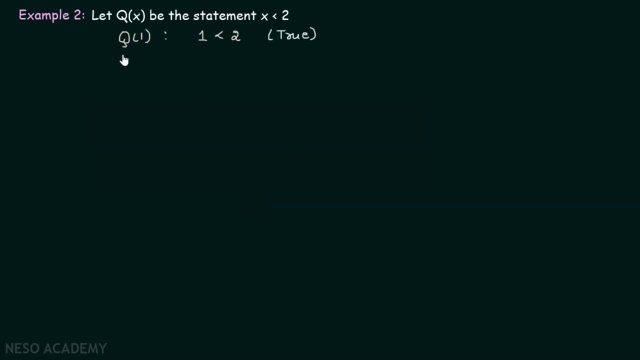 1 is less than 2, right, So definitely this is true. But if I ask what is the truth value for Q2? Then you will say: this is false. 2 is not less than 2.. This is false. 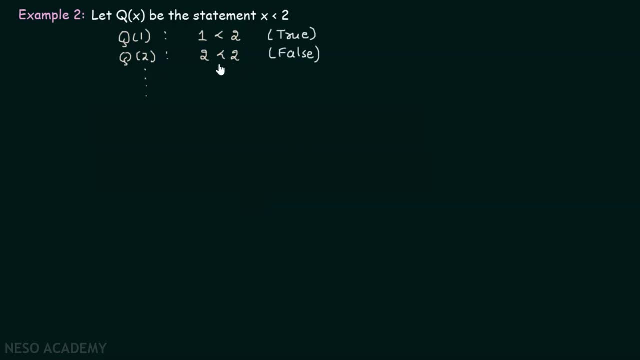 And if you take Q3, Q4, Q5 and so on, for all of them this will be false. This will only be true for this Q1. And for the rest of the positive integers this will be false. So my question is: is there some value of x?